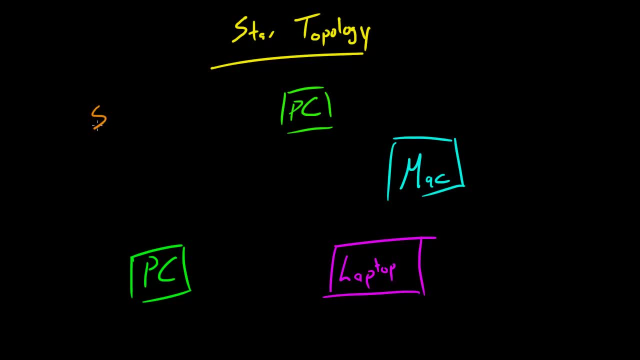 a personal problem coming out there And you also have a server- Not, you know, a waiter or anything like that, just a regular server- And in the middle this is how it gets the name: star topology. So what is a star topology? Well, basically, it's many different nodes or main, different devices connected to a central device. Now, the central device is usually something like a switch or a router, If you know Time Warner and came and set up a router. 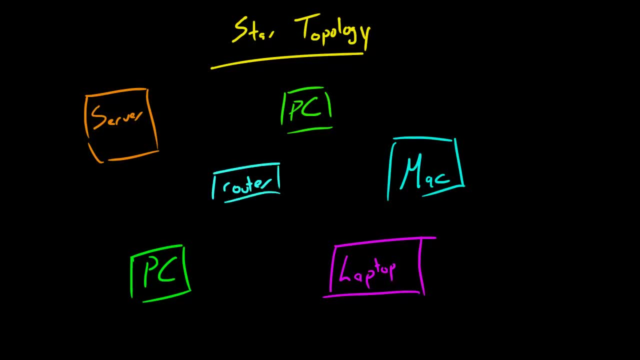 and then you took an Ethernet and connected all of your devices to it. like everyone's PC, everyone's laptop. we'll say that this laptop is actually, you know, has a Wi Fi card in it, And also the Macs usually have a Wi Fi card built in. But basically all of these different nodes are connected to a central device right here And, as you can see if you kind of squint your eyes and look, this kind of has a star shape because it has one central device. 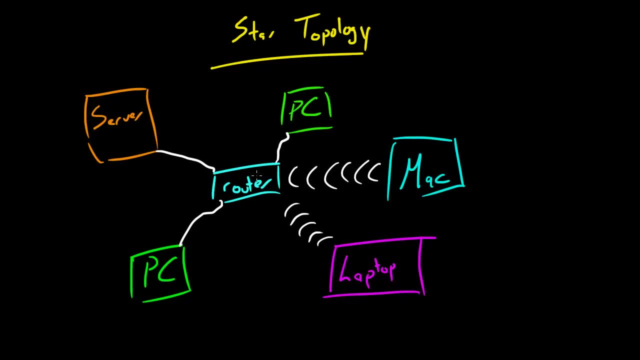 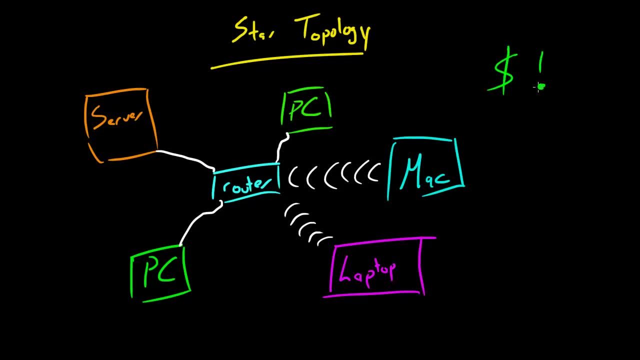 is really low. so cost is definitely a plus. and why is the cost really low? well, it's really easy to manage routers, since you know everyone is having the internet right now. they're made in bulk, they aren't really expensive and anytime you want to get, you know, an ethernet cable or a new computer, that's your cost, it's. 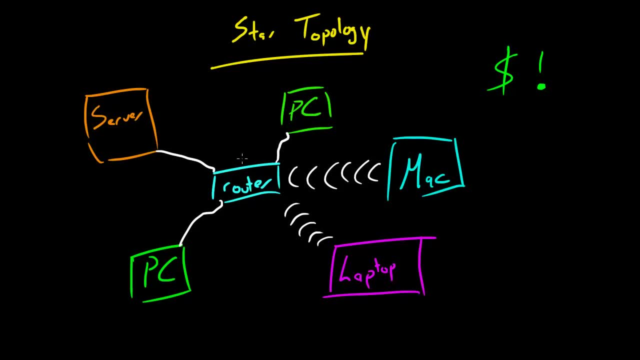 no cost of Time Warner, and if you decide to set up your own network like this, it's very cheap just to buy one single router instead of a bunch of different. you know random equipment now. another benefit of this is it's very easy to expand. if you know um, we'll say you only have one PC at first and then you know. 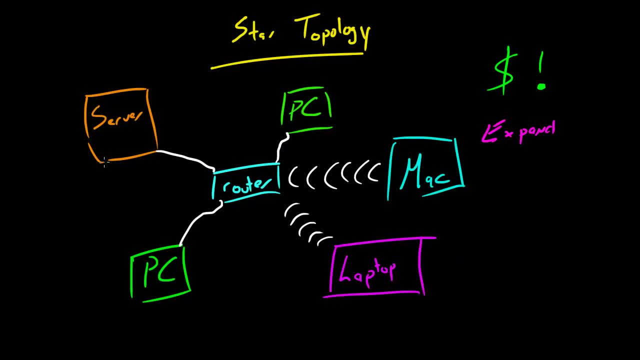 your girlfriend moves in with you and she has a laptop. and then, you know, your brother just got, you know, fired from his job and he moves in and he has another PC on your router. you have a lot of different ports so you have, you know, very easy expansion whenever you want to grow. 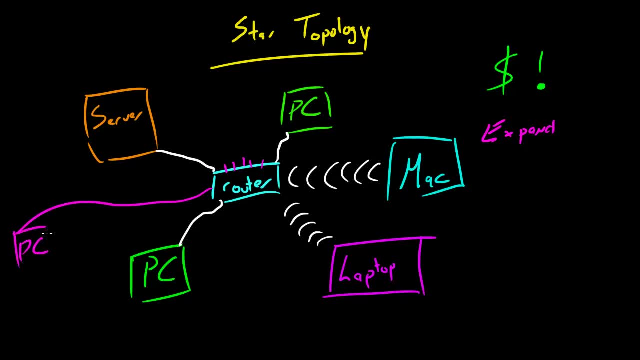 this network. you're going to have a lot of different ports, so you have, you know, very easy expansion whenever you want to grow the network, if you want to stick another PC on here. BAM, look at that, just did it in like 10 seconds. so those are the benefits of, you know, a star network, or? 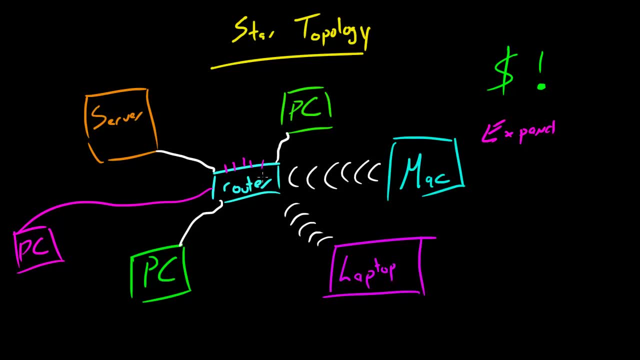 start topology rather than a bus or, you know, maybe a ring topology can be kind of confusing or expensive. and the last thing that I want to point out, which I should have mentioned earlier, is that another reason that people like this so much is because whenever one node I don't know goes down, maybe you have a 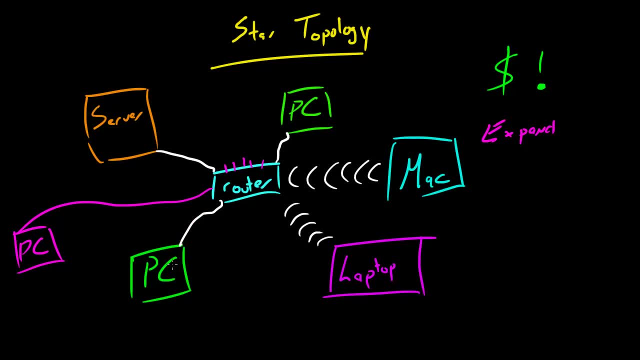 break in the ethernet cable right here because your dog ate it or maybe your PC got a virus. so this is kind of, you know, messing up the system. the rest of the network still works. it doesn't affect the router, it doesn't affect your server or anyone else's PC. 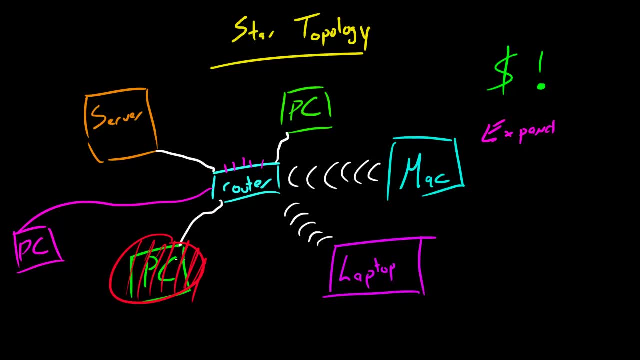 and that's why not only is it easy to fix, but it's also easy to identify and, unlike before, where this was a crucial part of the network, this can go down. you can even sell it or remove it completely and the rest of your network right here. 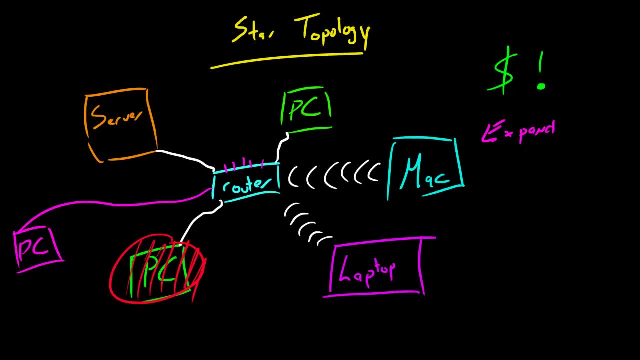 is going to work just fine. now, saying that brings me to my next point, which is the downside of this, because I just, you know, kind of talked on the benefits of this, but there actually is a downside to this and if you look, since everything is connected to this one central device, your entire network is dependent on this should. 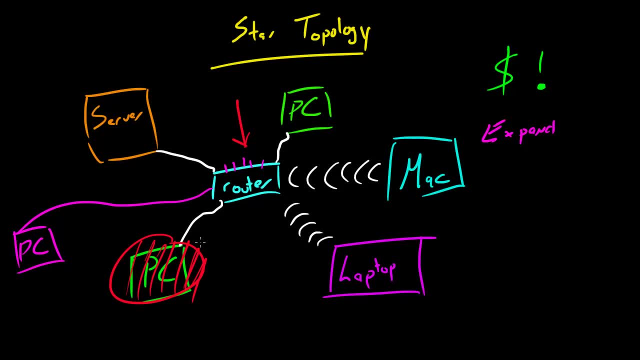 probably make an arrow on this router right here. so that means, unlike before, with, you know, our ring topology, our double ring: whenever this router goes down, every single computer is no longer able to access the internet. so that's one negative part about this: that every node is dependent on one single central device. and if this